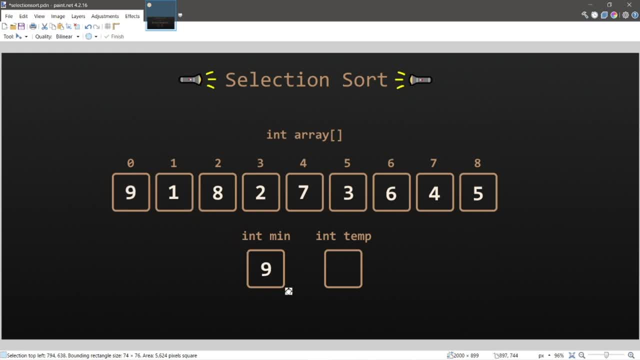 So we will move this value to some temporary storage. We'll keep track of the index of the minimum value. Nine is the new minimum. Let's open the next box and, holy crap, it's a one. One is a really small number, so that will be the new minimum. Then we'll open the next box. 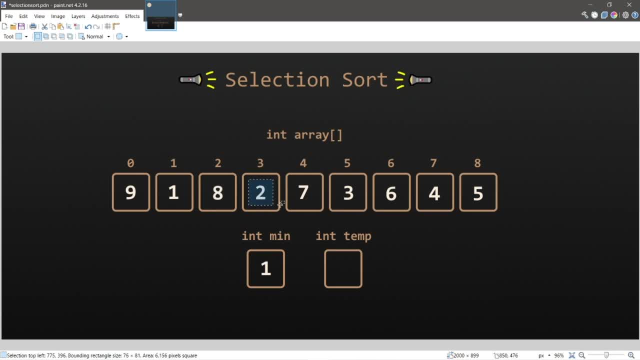 which is an eight. One is still less than eight. Let's move on. The next box is two, seven, three, six, four and five. One was the minimum value during this iteration and we need to move this value to the place that we started during this iteration: index zero. So we'll have 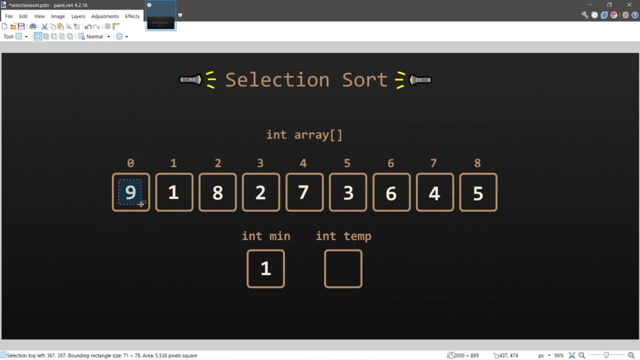 to do some good old variable swapping. So we will take nine, place it within some temporary storage, then take one and place it where nine was, Then take nine and place it where one was. And that is the first iteration. Let's move on to iteration two and we'll clear min and temp. 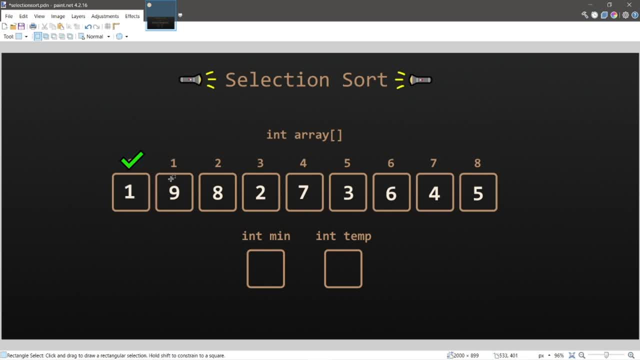 Okay, so this portion is done now We're not worried about it. This is the new beginning of the next iteration. and well, nine is a low number. I guess We'll move that to min. but eight is even lower than nine. 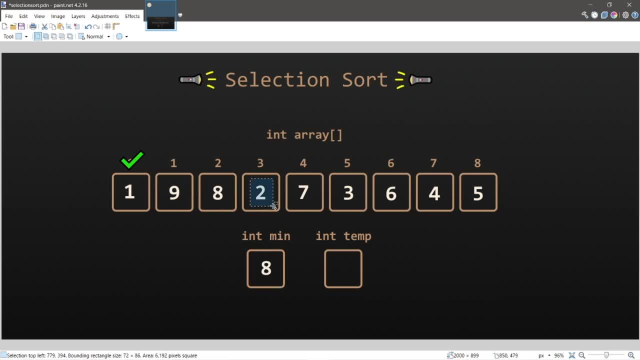 So we'll move that to min. Holy crap, it's a two. Two is the new min, for sure. And then we just repeat this process over and over again. Two is the current minimum of this iteration. One was the minimum of the first iteration, but we're not concerned with that. 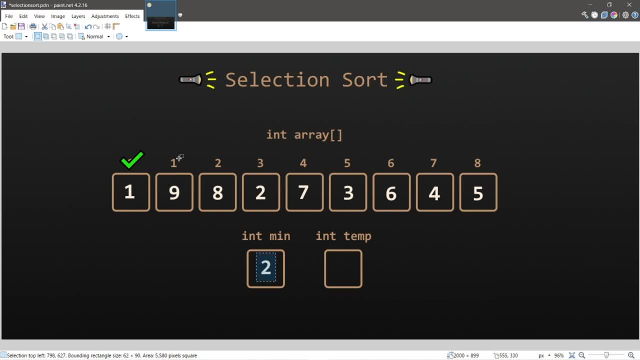 It's already sorted. So we need to move two to where we began this iteration, at index one, And currently there's a nine in there, so we're going to evict this nine. place it within some temporary shelter. take two, place it within. 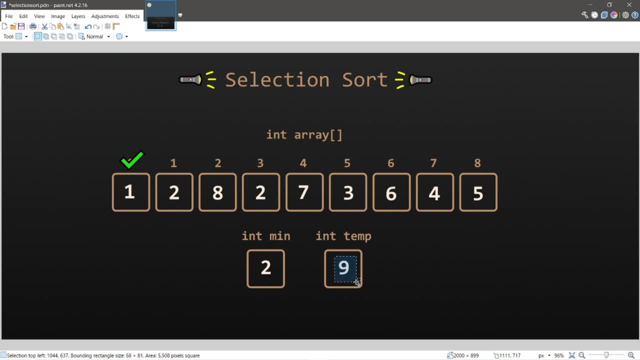 where we started at index one, then take nine, place it where two was, And that is the second iteration. Now that we kind of know how this process works, I'll speed up the rest of the video for this demonstration. So let's begin at index two. 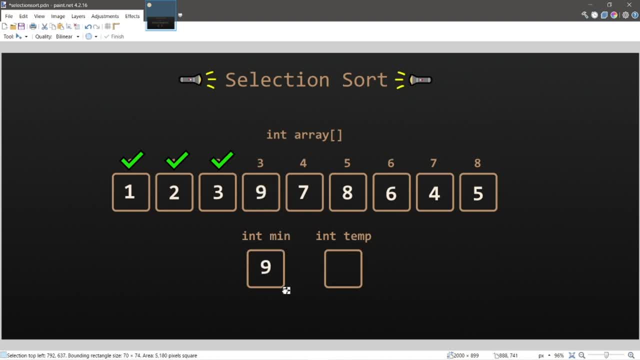 So that's index two, and that is index two, and that is index minus one, and that is index minus five, And that is this independence code. So now I'm going to open this up and we're going to see what the те r기를 is. 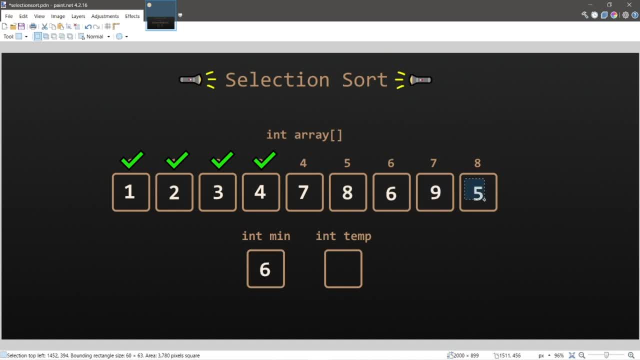 and then I'm going to run a more complex test. So my search method is this search method a little bit different because the query section here is independent? Thank you, And that is the Selection Sort Algorithm. The Selection Sort Algorithm has a runtime complexity of O of N, squared. 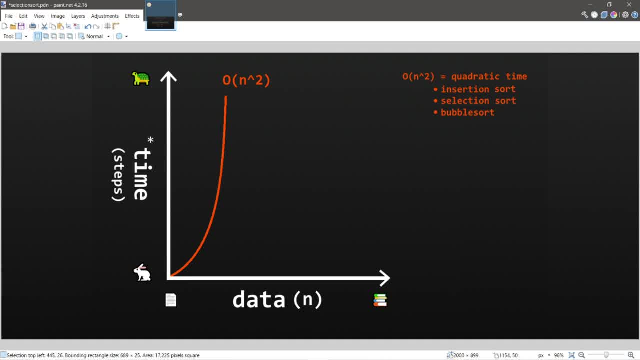 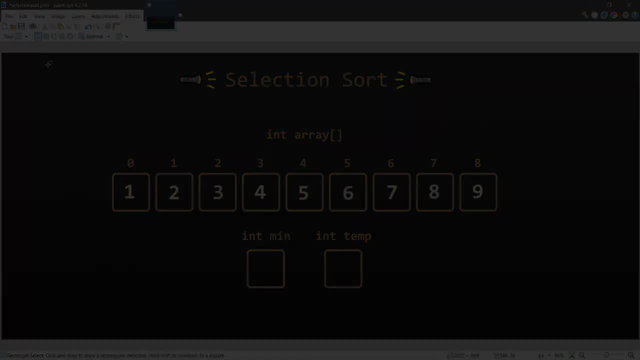 The larger the dataset, the more and more inefficient that using the Selection Sort Algorithm is going to be, Although it's okay with smaller datasets. Now let's create our own Selection Sort Algorithm. Okay, let's implement a Selection Sort. We'll need an array or other collection to work with. 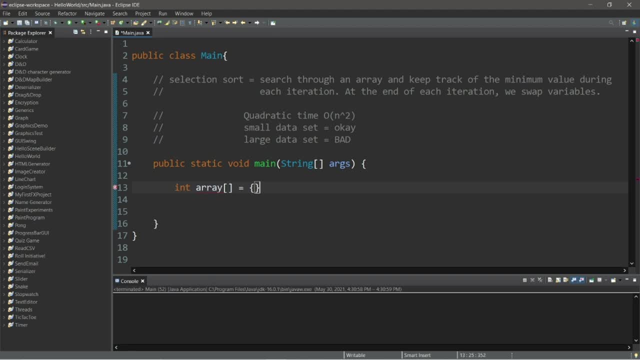 Let's create an array of integers, because I want to make this as easy as possible. So integer array and make up some random numbers. Make sure that they're not in order. What about 8, 7,, 9,, 2,, 3,, 1,, 5,, 4,, 6,, I guess? 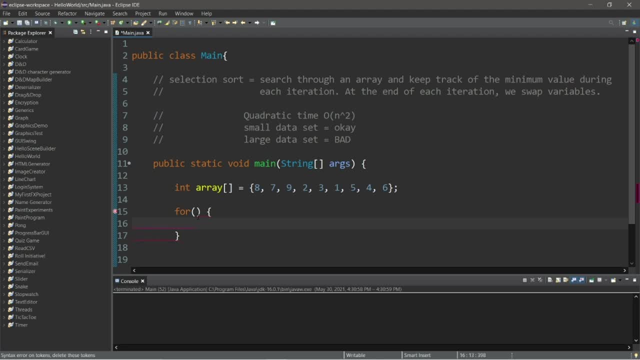 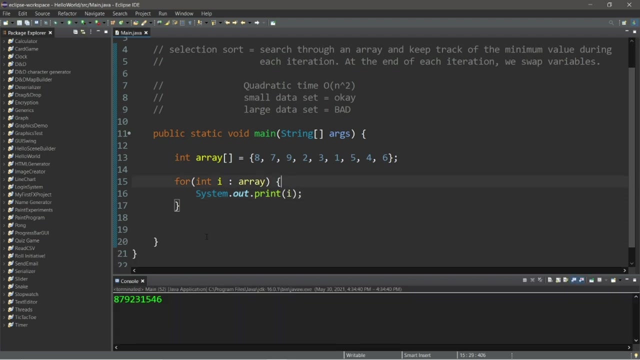 Then let's use a for each loop to iterate over the elements of this array. 4, int i In array. we will display each element with a print statement, Systemoutprint i. And let's run this once just to be sure that everything is working fine. 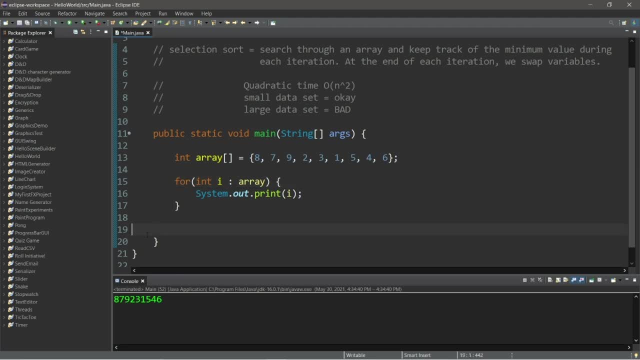 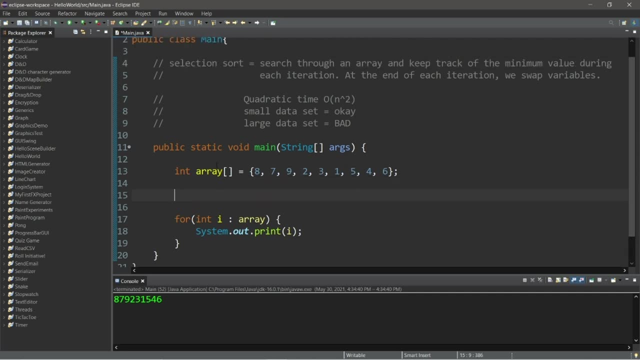 So 8,, 7,, 9,, 2,, 3,, 1,, 5,, 4, 6.. Everything is working as it should. So, before we display the elements of our array, let's invoke a Selection Sort function, which we still need to declare. 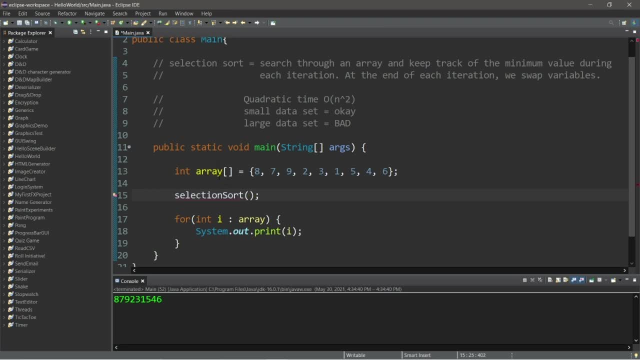 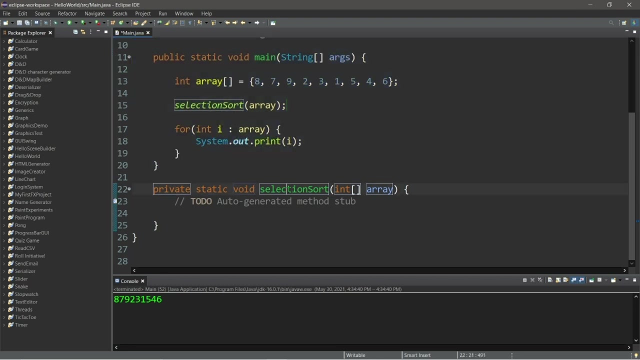 So Selection Sort And we will pass our array as an argument because, well, that's what we want to sort, right? So Selection Sort And we'll need to create this method. I will cheat and use the shortcut. So, outside of our main method, let's declare private static void. Selection Sort. 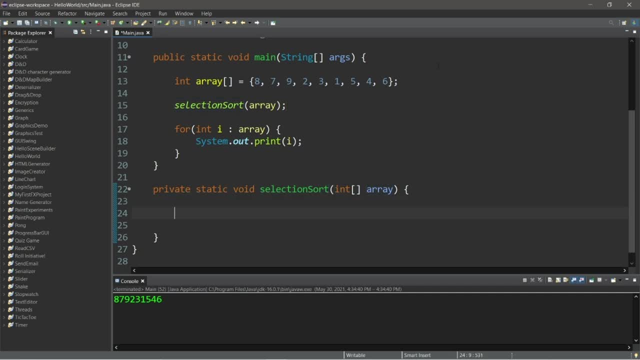 There is one parameter and array of integers. We'll need a pair of nested loops to iterate over our array, So let's work on the outer loop. 4, int i equals 0.. We will continue this as long as i is less than arrays length property minus 1.. 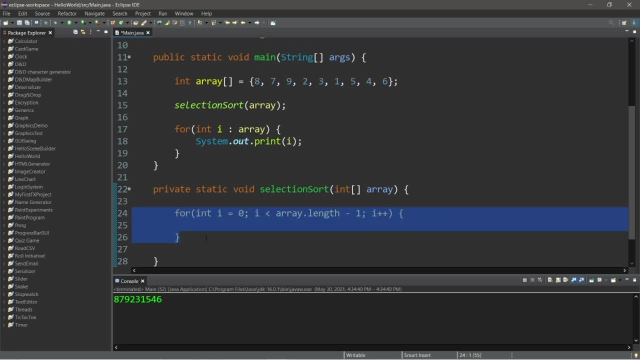 Then increment i by 1 during each iteration. Then there is a nested loop within here. Change i to j, So j equals i plus 1.. j is less than array length And j plus plus, So we'll need to keep track of the minimum. 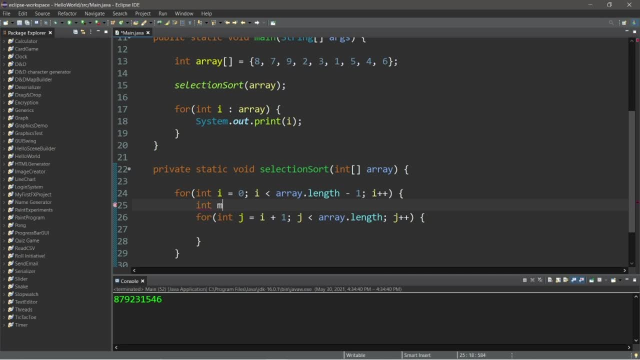 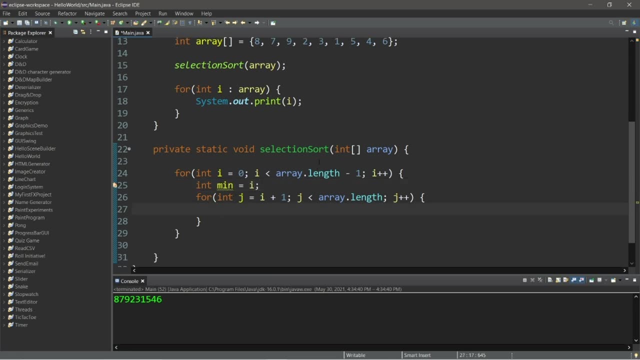 So we'll do that outside of our nested loop, int min equals i, So that is the current minimum, And within the nested for loop we will check to see if our array at index of min is greater than array at index of j. 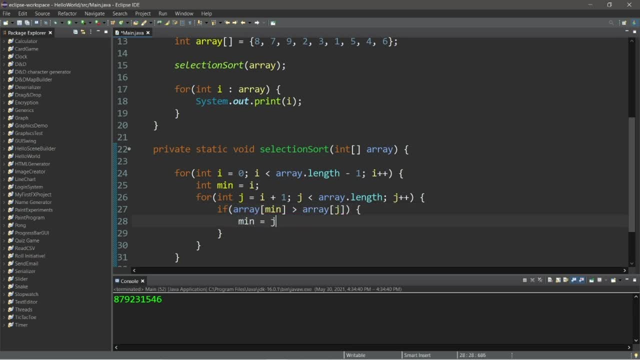 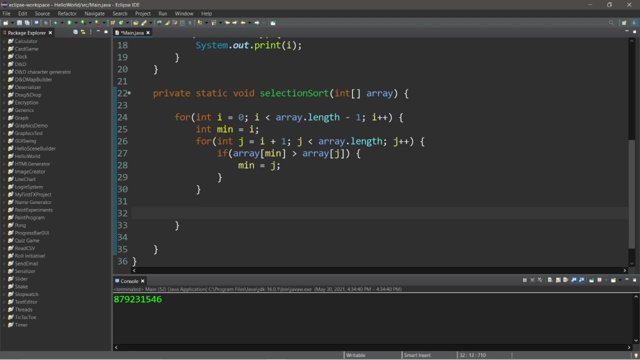 If it is, we will change our min to equal j. Then outside of our nested loop, but within the outer loop, we will do some good old variable swapping. So int temp equals array at index, Array at index of i to store this element. 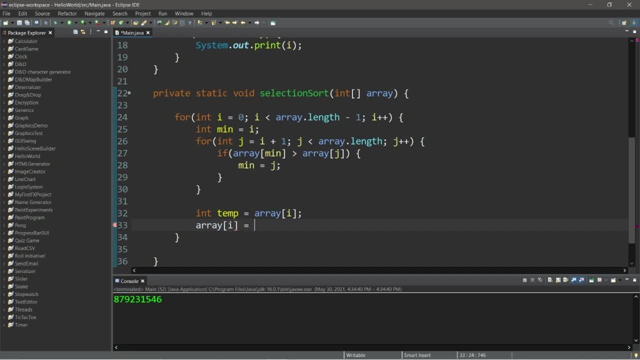 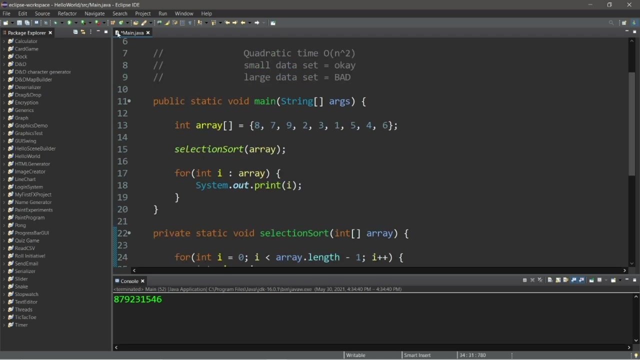 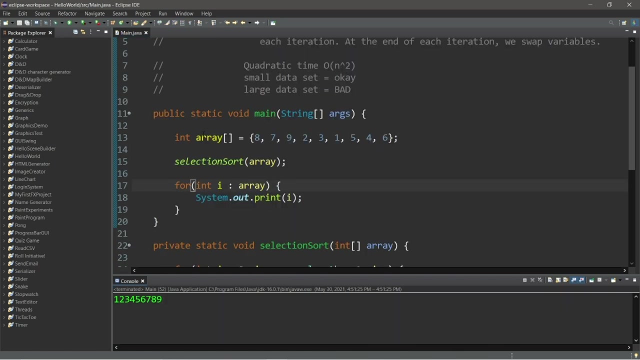 Array at index of i equals array at index of min. Then, lastly, array at index of min equals temp, And that's all there is to it. So, after running this program, our array is now sorted via the selection sort algorithm. Then, of course, if you need your array or collection sorted, 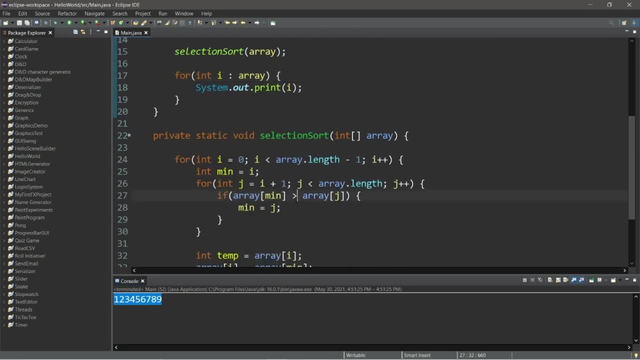 the array is sorted in descending order. Currently it's in ascending order. All we do is swap this greater than sign with a less than sign, And this will now be sorted in descending order, depending on what you need. Well, okay then, everybody.